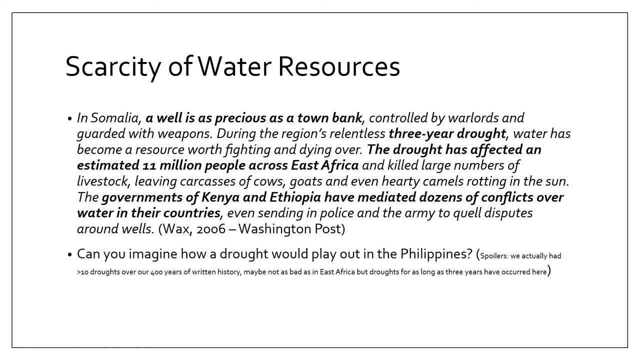 I had a friend who was from Kenya and he was studying water resources and we had subjects or courses that tackled water resources and he always commented how different it was in back in Africa. Like, for example, if you go to the water resources website, you will see a lot of water resources. 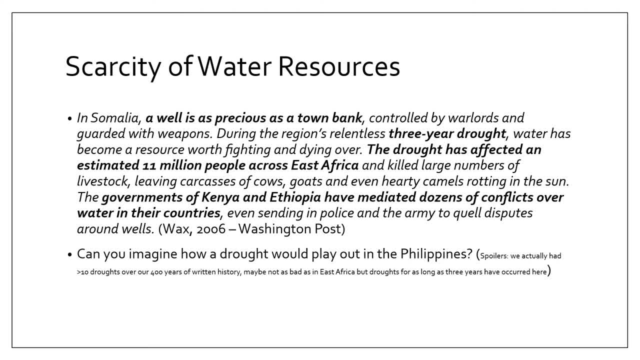 Like, for example, if you go to the water resources website, you will see a lot of water resources. For example, in New Zealand, they define water crisis as something like in the levels of their lakes being polluted by farming, while in Africa, their definition of water crisis is 10. 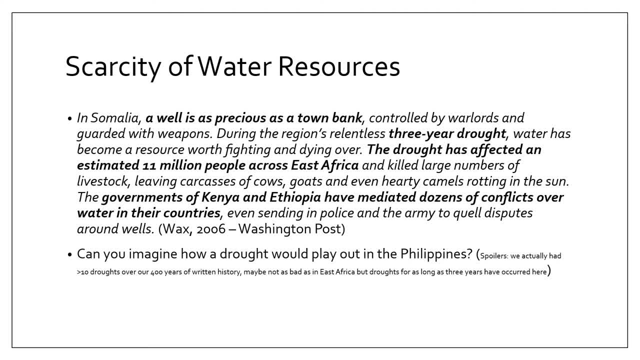 million people dying due to drought. I saw that stark contrast, so might as well read this excerpt. For example, in Somalia, a well is experienced as plant exposed novae for heating just three weeks to clean up戻 or a groundwater well is as precious as a town bank, controlled by warlords and guarded with. 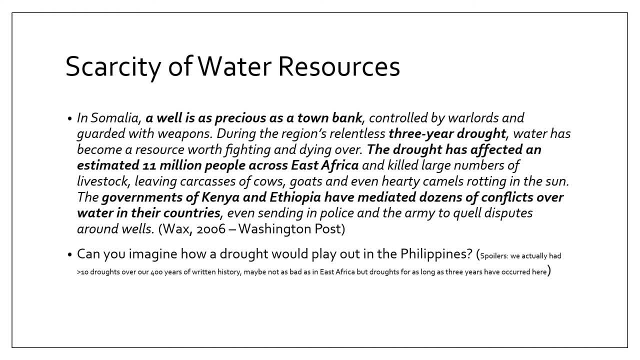 weapons. during the region's relentless three-year drought, water has become a resource worth fighting and dying over. the drought has affected an estimated 11 million people across east africa and killed large numbers of livestock, leaving carcasses of cows, goats and even hearty camels rotting in the sun. the governments of kenya and ethiopia have mediated dozens of 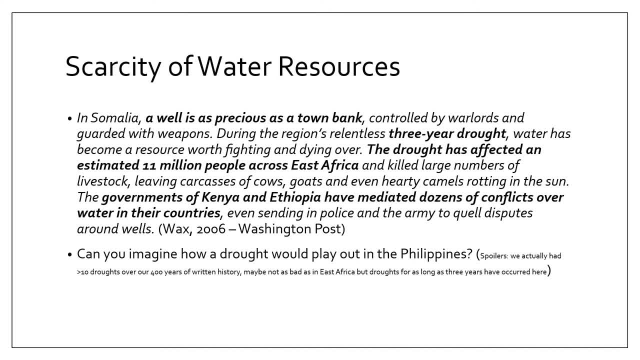 contact over water in their countries, even sending in police and army to quell disputes around wells. now, going back, so we are in the philippines. we are surrounded by sea and rivers. you may not be able to imagine how this relates to the philippines. okay, uh, surprise, surprise you. 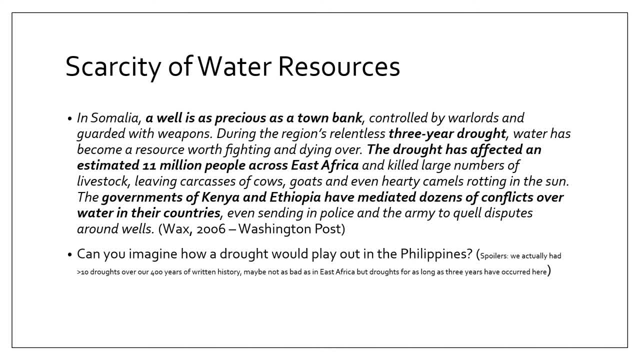 actually had droughts. i mean historically we had droughts in the philippines. although it is localized, meaning it, it. we had droughts before and they occur over over provinces, right right, and we had numerous jobs like almost, uh, over 10 droughts and over in the 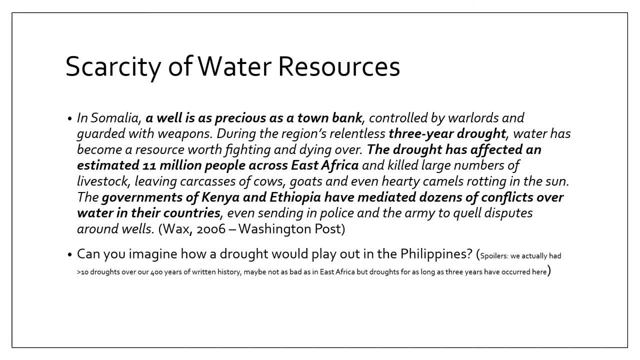 recorded history of the philippines and the longest one have have spanned as long as three years. okay, so that that's a big deal. i mean, you can imagine the recent water shortage in metro manila back in december 2020, and it was a pain in the ass to have. 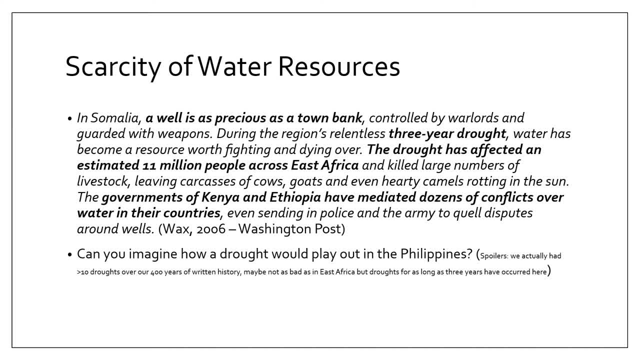 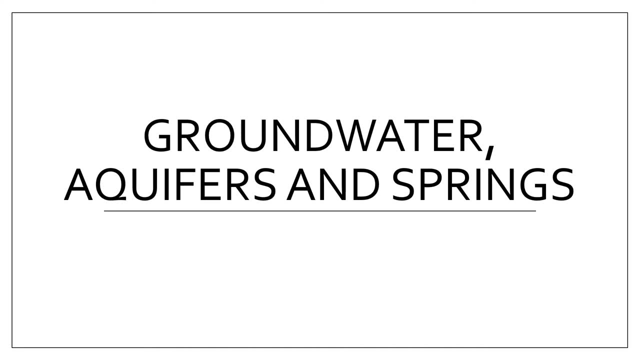 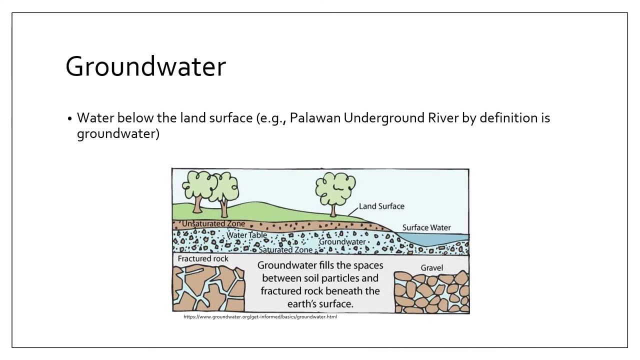 uh, or to deal with the low water pressure, and you can imagine having that problem: having no water for three years. okay, all right, let's proceed to the uh first part of this module, the groundwater, aquifers and springs. groundwater is essentially water below the land surface, by definition, the palawan underground. 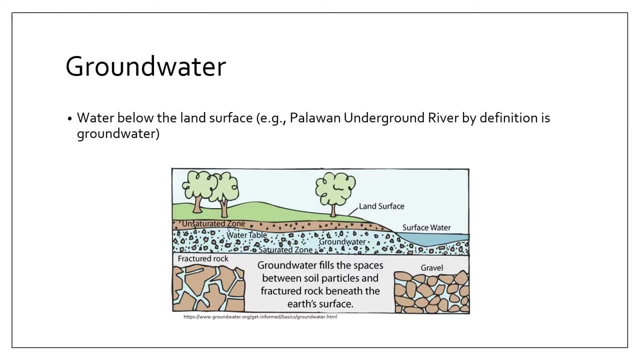 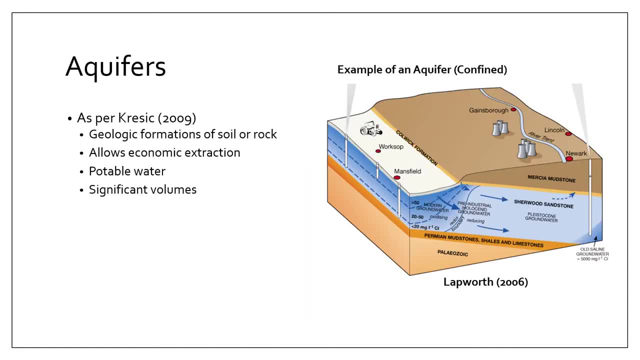 river is groundwater, so any water that is below the land, below the land surface, is groundwater. now, aquifers, as per cresic 2009, consists of geologic formations of soil or rock, and the key keywords here are economic extraction, potable water and significant volumes. now you will realize that definition, that the definition of aquifers. 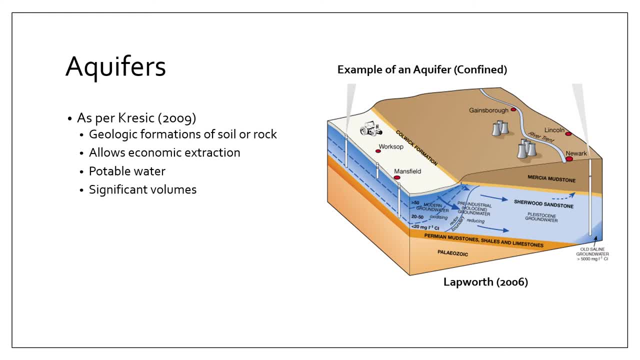 is quite similar to the definition of ore minerals, in a sense that it is a relative definition. okay, so we peg the definition of aquifers to the economics of it. so any water that can be economic, economically extracted and is potable and insignificant in volume is technically an aquifer. 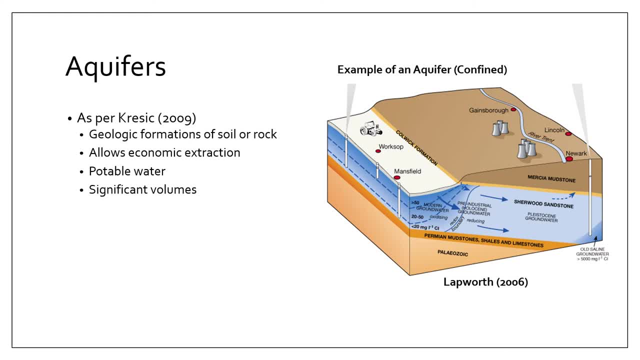 right, and you can see an example here right showing a block diagram of an aquifer. in this case, the aquifer is a sandstone, the sherwood sandstone, and it is overlaid by a mudstone later than. it is underlined that the ak���. 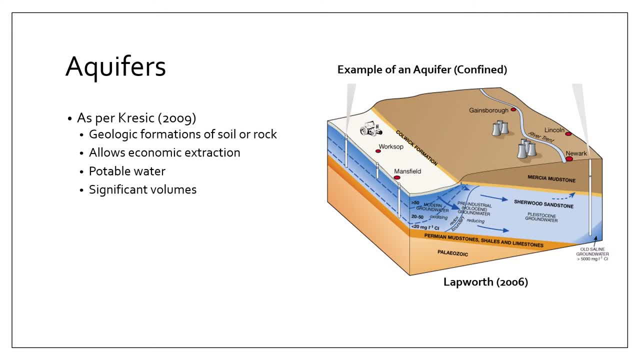 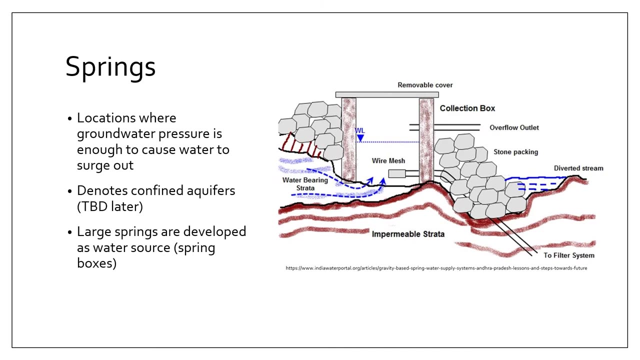 is permitted and has its underlying bedrock is permian mudstones. okay, note that the aquifer has a confined aquifer because it has a confining layer on top. now, springs are locations where the groundwater pressure is enough to cause your water to surge out. okay and typically. 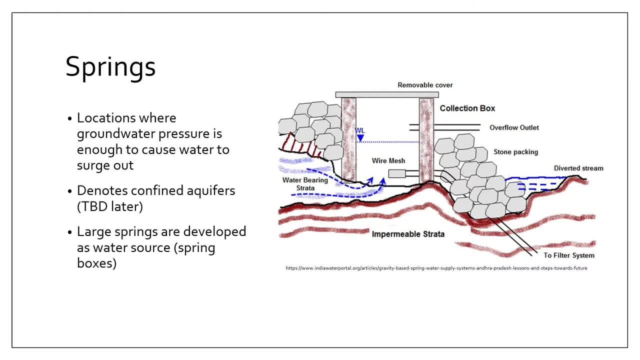 yet you have springs when you have confined aquifers in terms of water supply, springs, or rather large springs, are important as they can be developed as into a water source by the construction of spring boxes. the diagram here is a schematic of a spring box and the diagram here is a schematic of a spring box. and. 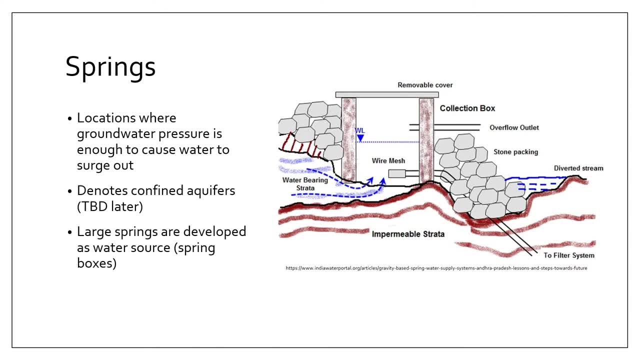 right. you can see here you have a housing, typically made of concrete, which impounds spring water and it collects water from a connected water bearing strata right, and then you also have a filter system for water that is diverted into to your households or to your farms, whatever it is, and you also have 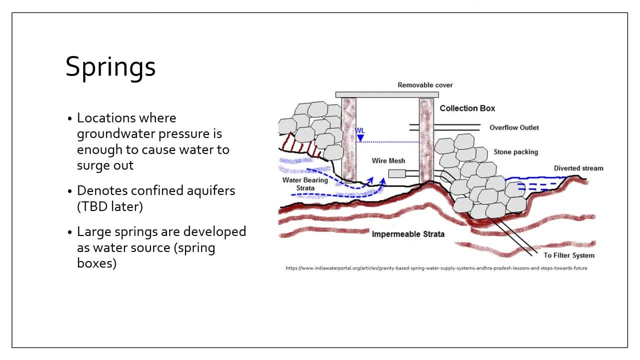 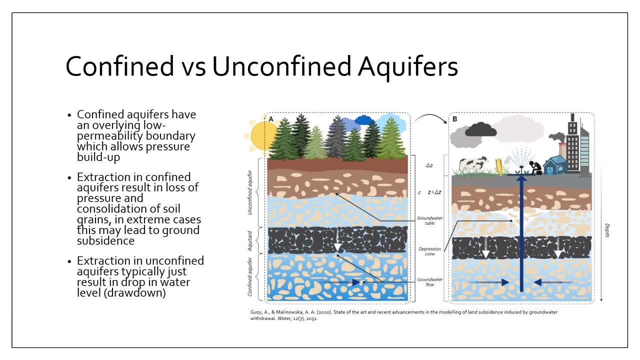 an external collection access, or so you can access the spring box from the outside, okay, and it also has a cover to protect the spring from contamination from out, from outside. now let's define confined and unconfined aquifers. confined aquifers have an overlying low. 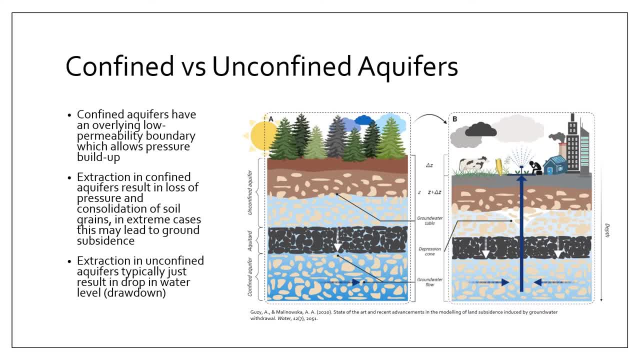 permeability boundary or a low permeability formation, and this confinement allows pressure build up. right, because as you accumulate water in an in a confined aquifer, the water basically can only move laterally. it can't move upward anymore because it has a confining layer, so this results in pressure buildup. 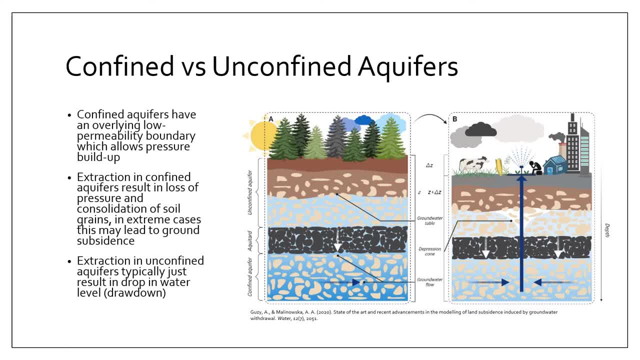 right now for confined aquifers. when you extract water, what happens here? what happens is you reduce the pressure in the confined aquifer and, as a result, okay, the loss of pressure results in your soil grains within the aquifer to stick together and possibly consolidate- okay, depending on the severity of the loss of pressure in extreme. 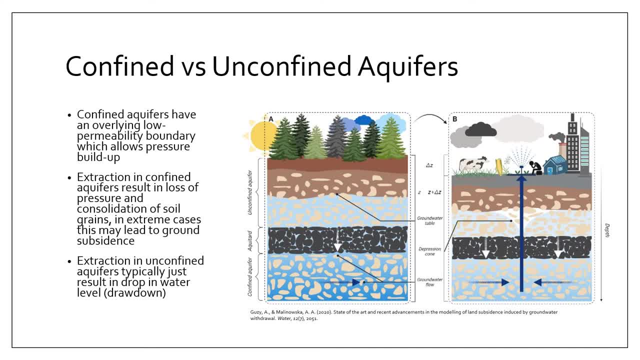 cases where there is a vigorous extraction of ground water in your confined aquifer, this can lead to ground subsidence. okay, and the thing with confined aquifers is you can imagine confined aquifers as a bladder of water- okay, and as you squeeze out the water- okay, if you squeeze out a significant amount of water- the bladder just loses water and it sort of 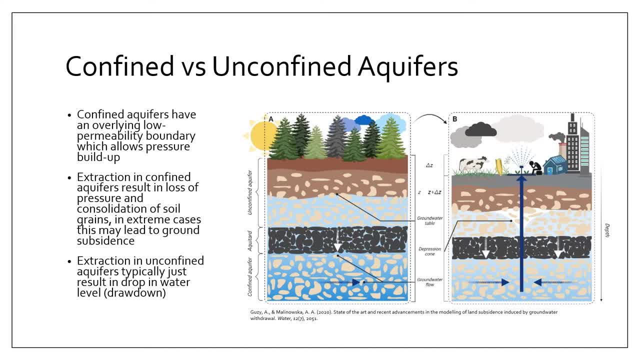 shrinks in size spread out all the time, and then it is noticeable that they sink and that they become too big. confined aquifers generally do not easily recover or they sometimes they permanently loose, they permanently undergo subsidence. now, in the case of unconfined aquifers, which are generally open, 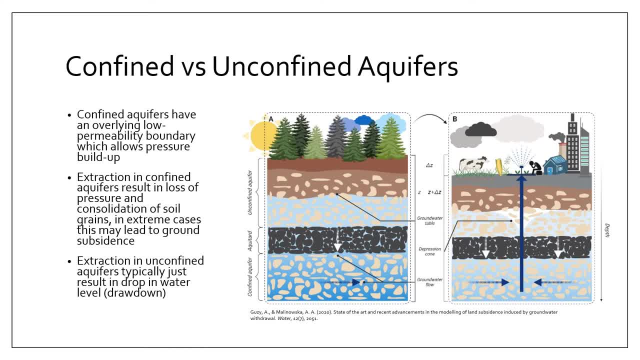 okay for the case of unconfined aquifers, which are still open for extraction. during those times, humans can have no need for water pointed areas" and unconfined aquifers typically just result in drop in water level. As you can see in the diagram here, this is a good representation of a confined aquifer. In some cases, the water 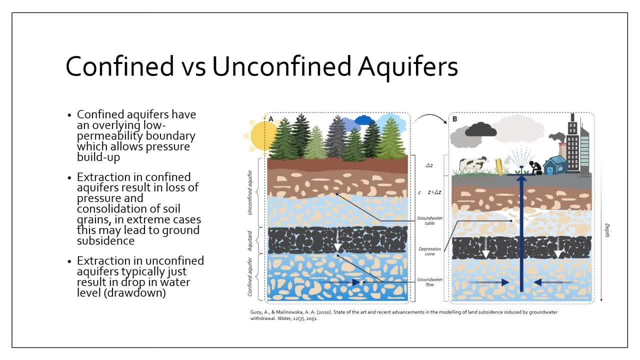 pressure is large enough such that the soil grains in the confined aquifer are hardly touching, meaning the soil skeleton or the soil skeleton structure is hardly supporting the weight of the overburden above, Or in other words, there are confined aquifers where you have so much pressure. 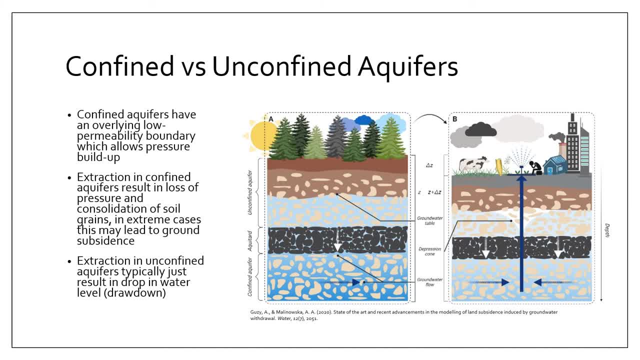 that parts of the overburden is being supported by water pressure. Now, when you extract the water from that confined aquifer, you start taking out water pressure and, as a result, you slowly transfer the load or the overburden to the soil grains and that results in consolidation for soft soil and soil structure. 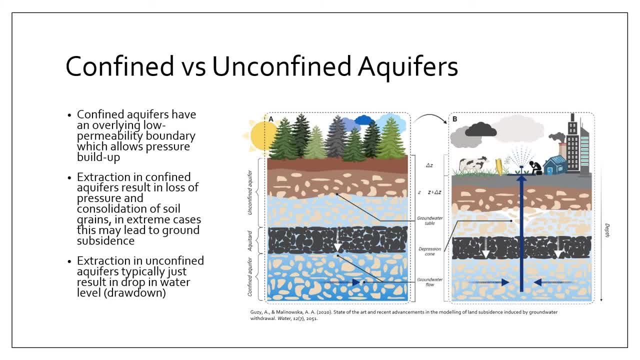 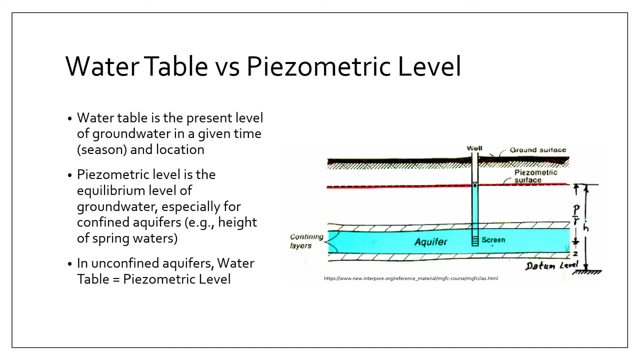 compaction for granular soils. okay, and it can be permanent. okay, could be a permanent, permanent effect for the confined aquifer. now let's let's differentiate water t-ball versus piezometric level. water table is simply the present level of groundwater given a time and a location. right. note that water table fluctuate. 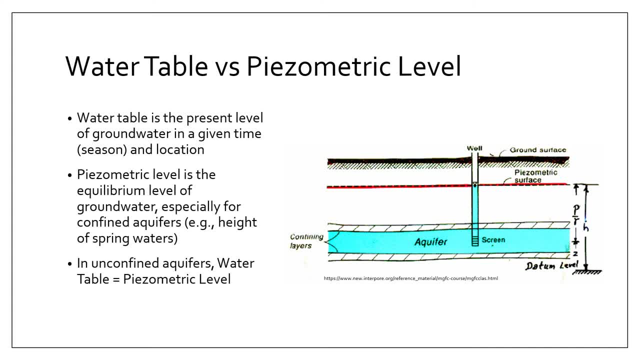 fluctuates with your season, especially dry and wet season, you get water table fluctuations. in a sense, water table is just the literal water elevation of your water- okay- while piezometric level is the equilibrium level of your groundwater, particularly for confined aquifers- okay. in the case of unconfined aquifers, water table is just the same as piezometric level. 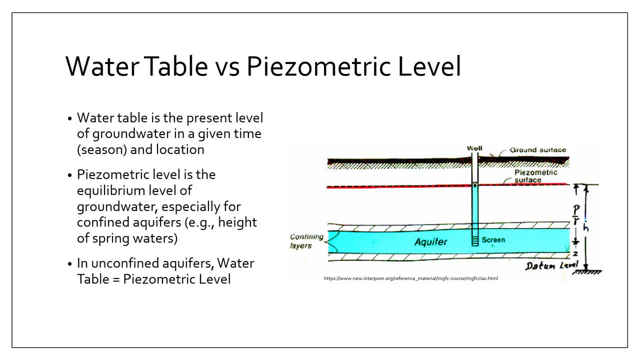 and for the case of of confined aquifers, the water level is often different from the piezometric surface or the piezometric level, as shown in this illustration right in this point, and you can see here the top level of top portion of the aquifer. here is the water table. 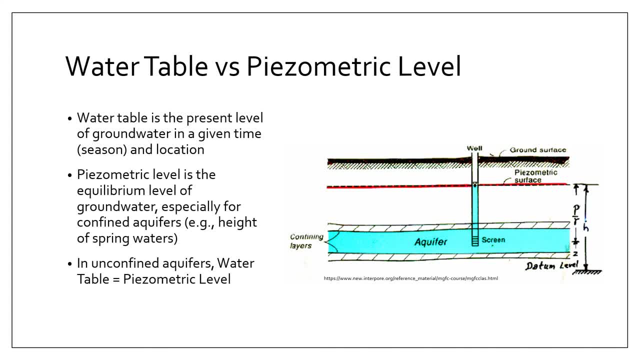 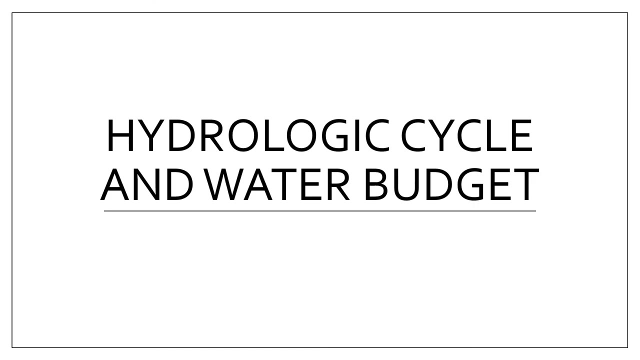 but the piezometric surface is actually well beyond, or well above your water table. now, once you introduce a well which allows the aquifer to release its pressure, your water can actually rise right well into the piezometric level. right now let's talk about hydrologic cycle and water budget. 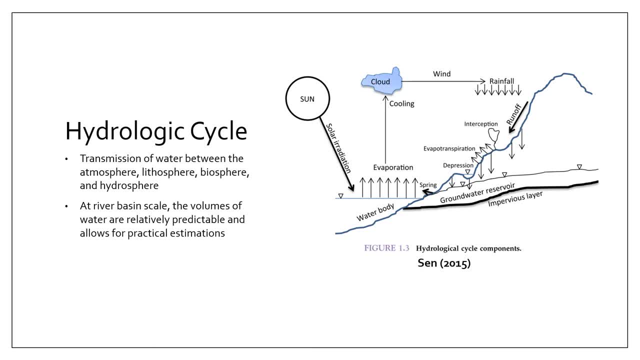 hydrologic cycle. this is basically how you, how water, is transmitted throughout your environment, and this involves the atmosphere, in form of your precipitation, and then your lithosphere, in form of runoff, being the being in form of your, your watershed transforming precipitation into runoff, as well as your biosphere. 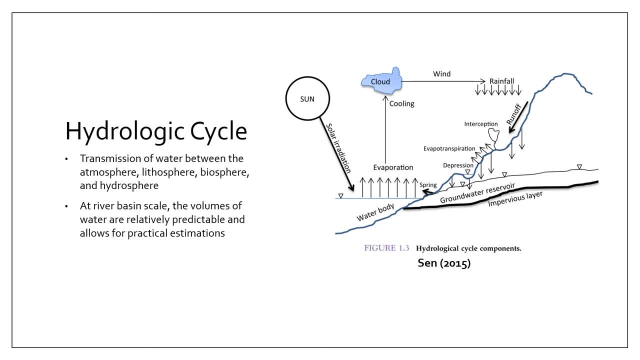 which involves the, the evapotranspiration of water from your plants and then to your hydrosphere, which involves the, the discharge of your, of your runoff to these, to the sea or to a lake, as well as the discharge of ground water into your rivers. 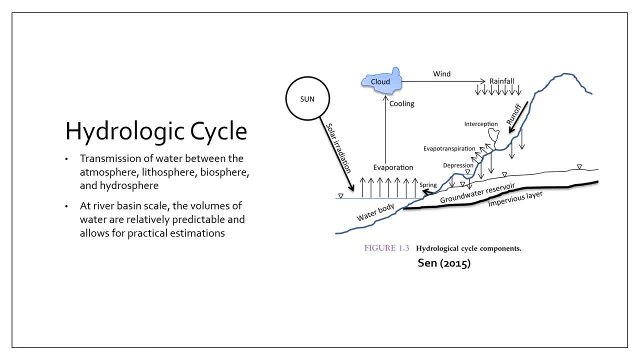 normally note that at a river basin scale or or at a watershed scale, the volumes of water ar relatively predictable and allows for practical estimations. why? because when you're looking at a particular river basin or a water basin, more or less the precipitation is the precipitation that lands in your 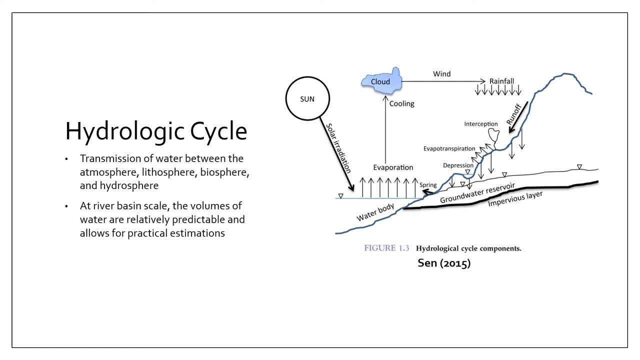 watershed, okay, has a predictable destination, so the rain in your watershed will turn into runoff and then it might infiltrate or it might enter your stream and then exit through the main outlet, which might go to the sea or to a lake. okay, you are more or less not losing a lot of water to, to an extent, the 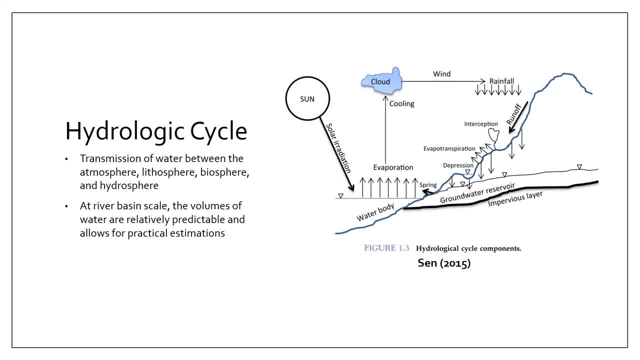 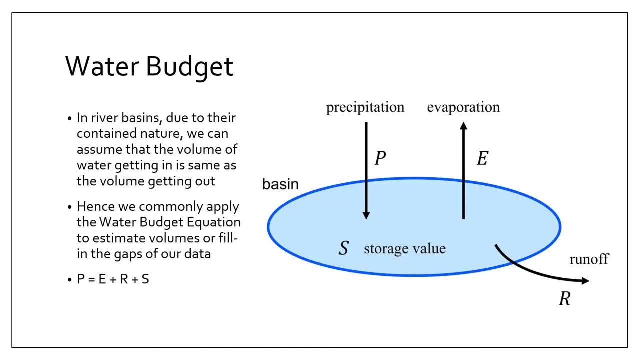 water is more or less not not going outside the boundary except for its defined outlets. okay, so, due to the contained nature of the watershed, the rain is not going out of the boundary except for its defined outlets. okay, so, due to the contained nature of river basins, we can assume that the volume of water that is getting in is. 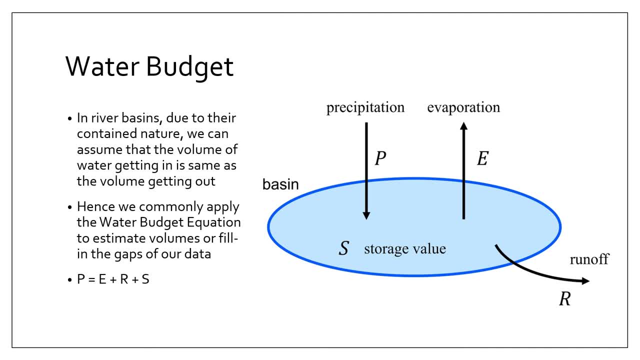 more or less the same as the volume of water that is getting out, and we can apply the water budget equation to estimate volumes or fill in the gaps of our data. now note that the water budget equation has many forms. it can be as complicated as the water budget equation, but it is a very complicated. 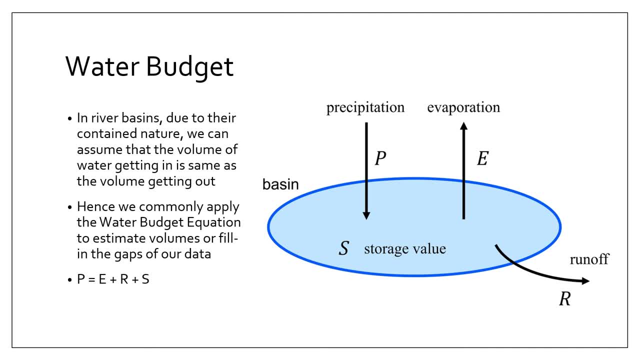 as including infiltration, base flow, shallow groundwater, deep groundwater water and so on. but for our purposes, we just want a simplistic introduction of the water budget equation. water budget equation is basically P, or precipitation is equal to evaporation, or sometimes evapotranspiration, plus your runoff and then plus your storage value of your groundwater right? so now let's. 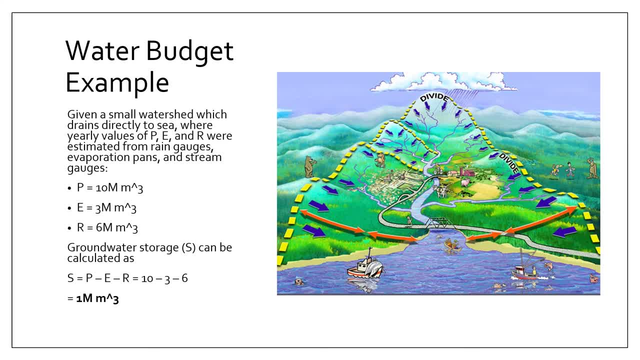 take a simple example. here we have a watershed, or a small watershed which directly drains to the sea, and we have the following values of your P, E and R, which were taken from rain gauges, evaporation pads and stream gauges. okay, so precipitation is 10 million cubic meters, evaporation is 3. 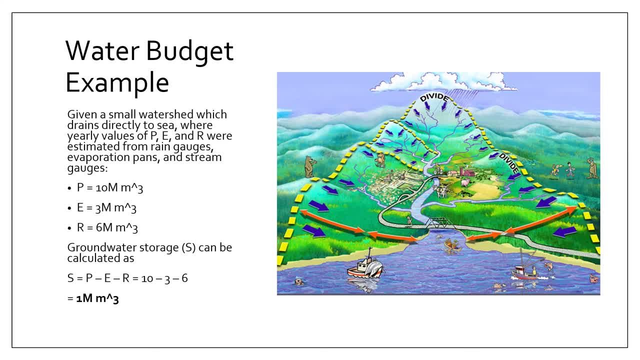 million cubic meters and then the estimated runoff is 6 million cubic meters. from those values we can estimate the groundwater storage as S is equal to P minus E minus R, which is 10 minus 3 minus 6, and that gives us a groundwater storage of 1 million cubic meter all. right.